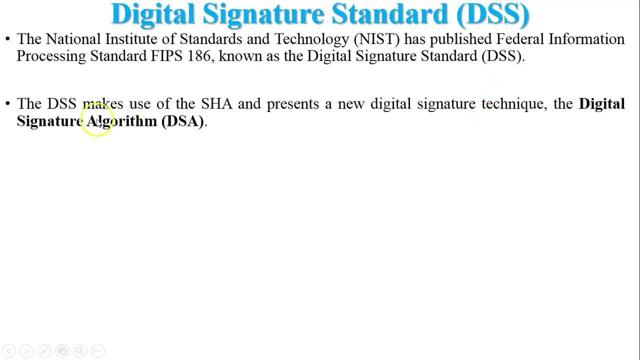 as the Digital Signature Standard. The DSS makes use of SHA and presents a new digital signature technique. the Digital Signature Algorithm Latest version also incorporates Digital Signature Algorithm based on RSA and Elliptical Cow Cryptography. Let us discuss about RSA and DSS approach. then later on we will discuss about DSA Algorithm. 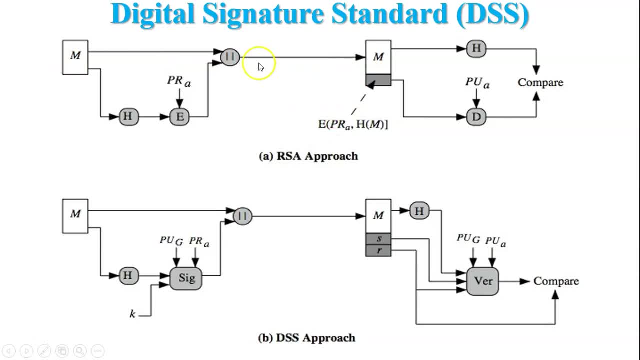 Now see this two diagram. so above diagram is RSA approach and below diagram is DSS approach. The difference of both the diagram is here: in RSA approach simply private key and public key concept is used. also hash function is applied In DSS approach here private key and public key. 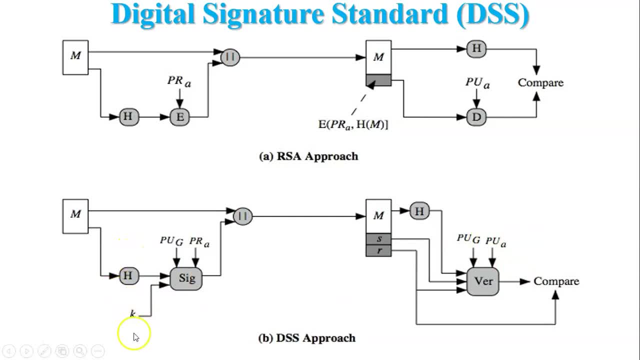 concept is used. also hash function is applied. also new secret key is applied and global component of public key concept is also used. Now see this two diagram. so above diagram is RSA approach and DSS approach. here private key is also used For the particular group of users communication. So 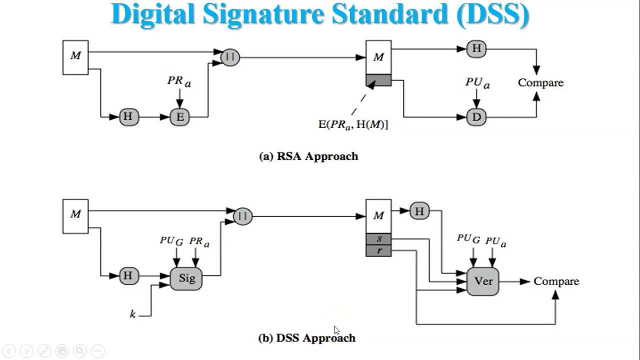 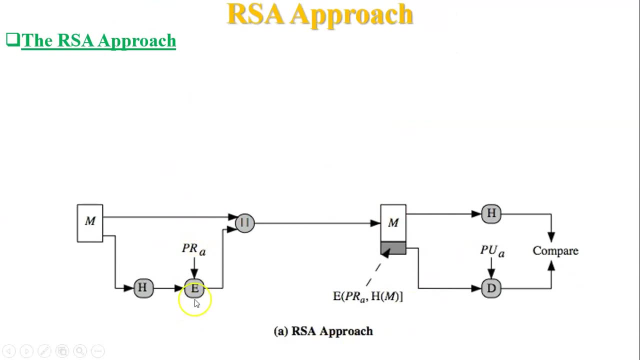 DSS provide more security in compared to RSA approach. Now discuss about RSA approach. So this below figure is shown for the RSA approach. First point: in the RSA approach the message to be signed is input to hash function that produce a secure hash code of the fixed length. So this: 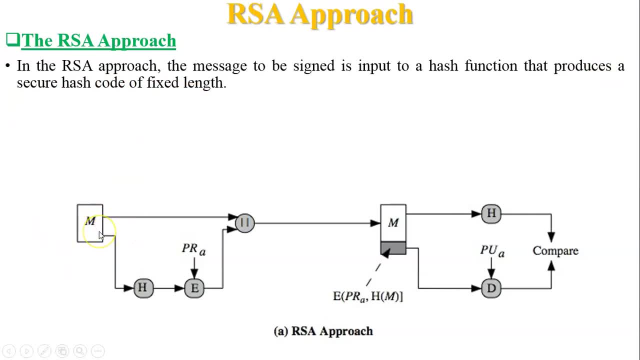 is the message at the sender side: Apply any hash function on the sender side: Apply any hash function algorithm. for example SHF1 algorithm, is used and it generates a fixed output. Here hash function is used and final output value is hash value. The hash code is then encrypted using the senders private. 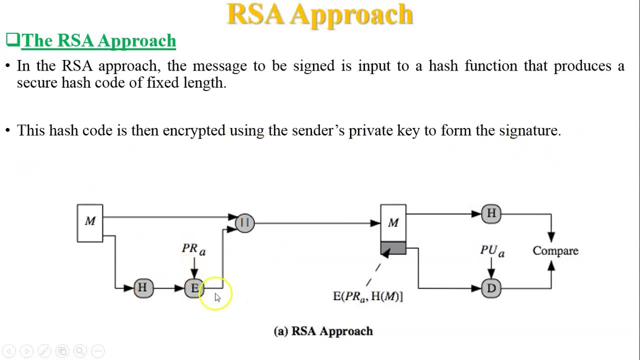 key to form the signature. Now you can see over here: this is the encryption of the hash function with the help of senders private key. Here for the decryption, senders public key is used. it means there is public key. So this is the decryption of the hash function. So this is the decryption of the. 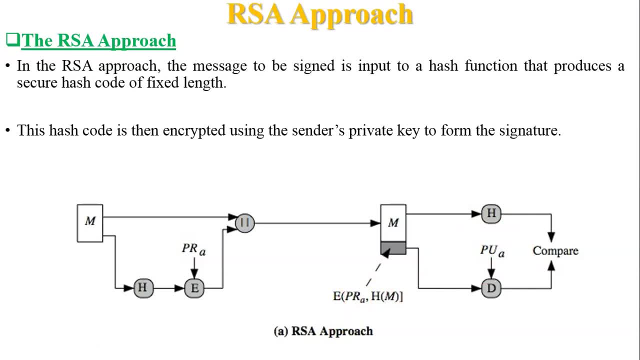 hash function. So this is public key cryptography used. we can say RSA approach is used and the encryption means to apply, or we can say to add for the signature, or we can say to check integrity and authentication during the transmission. Both the message and the signature are then transmitted. 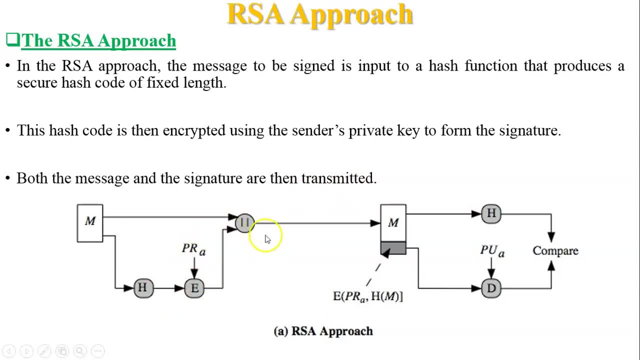 Now encrypted hash value, attached with the message and sent to the receiver side. The recipient or may or it may be receiver takes the message and produce a hash code. Now, in this figure you can see over here from the message, receiver will use the SHA1 or any kind of algorithm and generate hash function and it compares to the 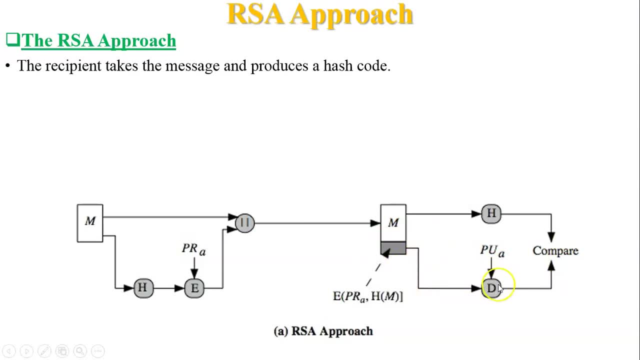 encrypted hash function. Here encrypted hash function is decrypted using the public key of the sender. This public key is shared by the sender with the particular receiver and decrypt and then compare with the generated hash function. If both are same, it means message is valid and accept by the particular receiver. 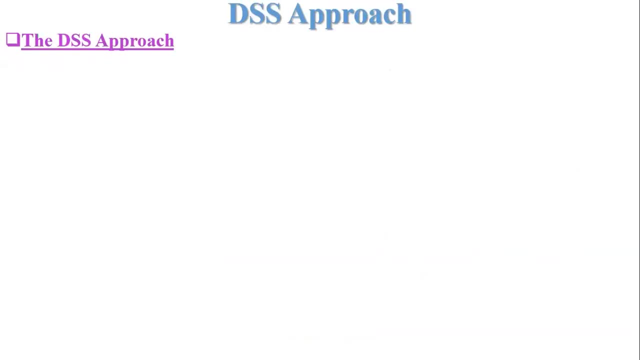 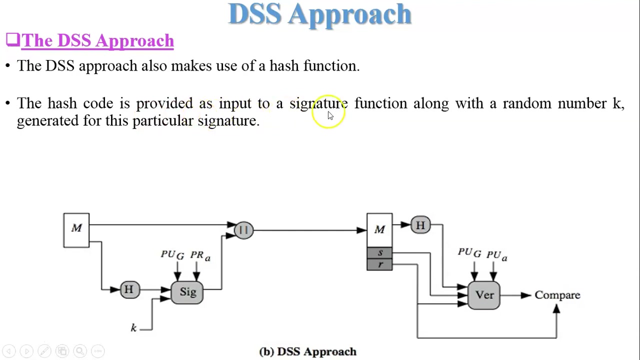 So this is the RSA approach. Now next is DSS approach. In DSS approach also make use of a hash function. Now see in this figure: this is the hash function. this is original message at the sender side. The hash code is provide as input to a signature function, along with a random number of k generated for the particular signature. 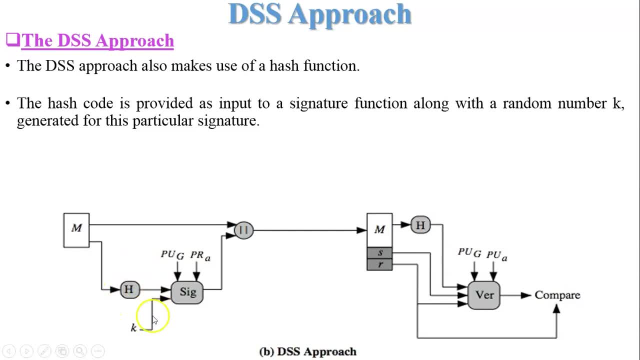 So signature is generated from the hash function. Here one variable, k, is added. Here the value of k is new whenever new message is arrived for the signature. Whenever your message will be different, the value of the k will be different every time. The signature function also depends on the sender's private key, PRA. 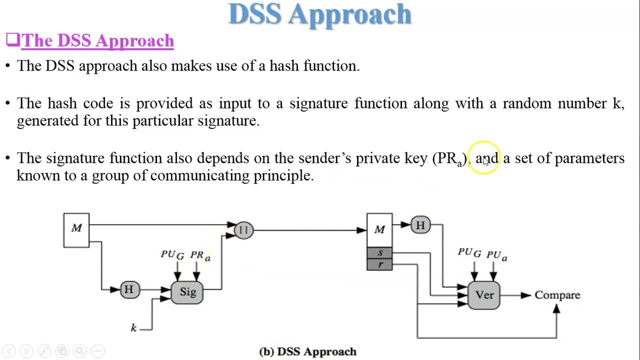 Now you can see over here. this is the PRA sender's private key And a set of parameters known to a group of communicating principle for the PUG Here, PUG meaning group of public key whenever more than two users or number of users are connected in the network. 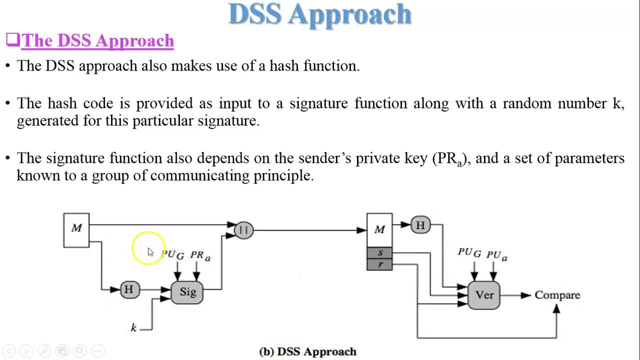 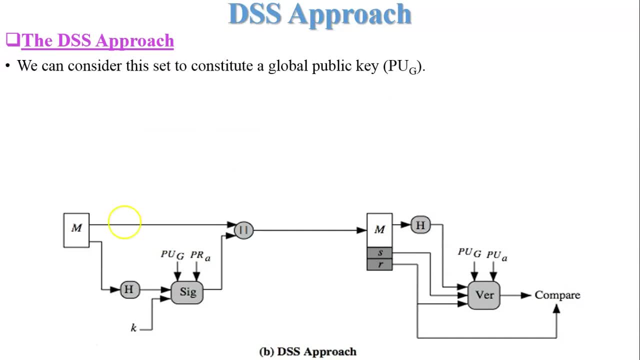 So here, PUG component, we can say global public key is same for all the users, that all are connected in the network. We can consider this set of constitutive of global public key And set of global public key is PUG. So the result is a signature consists of two components: level S and R. 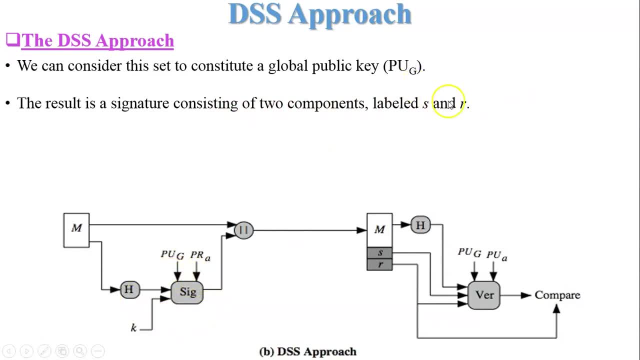 So we can say signature will be based on S and R. We can say the pair of S and R is the signature of the particular message and appended to the message At the receiver end, the hash code of the incoming message is generated. Now see over here: from the message hash code is generated. 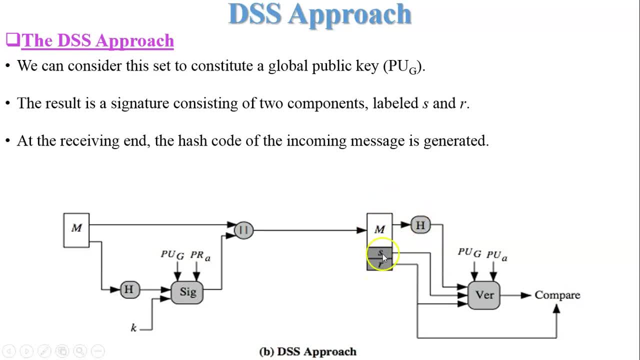 Appended S and R will be over here. This is the digital signature of the particular message generated by the sender. The signature is input to a verification function So we can say: signature will be verify with the particular receiver. If there is any forgery or there is any integrity in the message or signature is not valid. 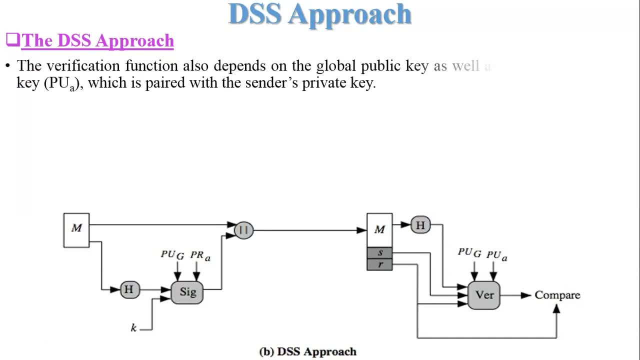 Message will not accept by the particular receiver. The verification function also depends on the global public key as well as the sender's public key, PUA. Now see over here. this is the verification function. Here global public key is used, which is used as the same sender side. 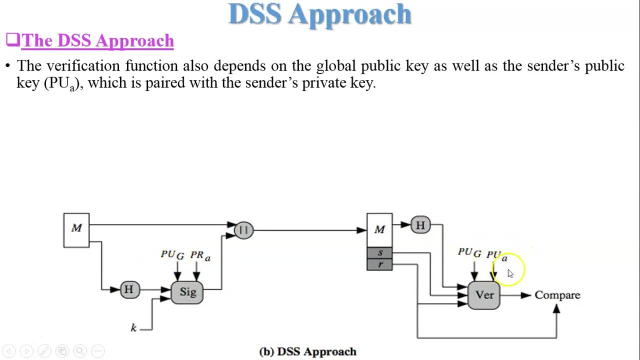 Here public key of A is used. Here, public key of A is shared by the particular sender, which is paired with the sender's private key. The output of the verification function is a value that is equal to the signature component, If the signature is valid. 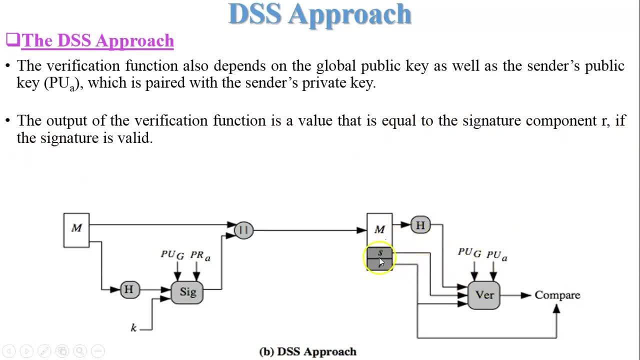 Now see over here from the M, S and R is input of the verification function. Also, global public key component and sender's public key is the input of the verification function and it generates value. The generated value from the verification function is same as the R. 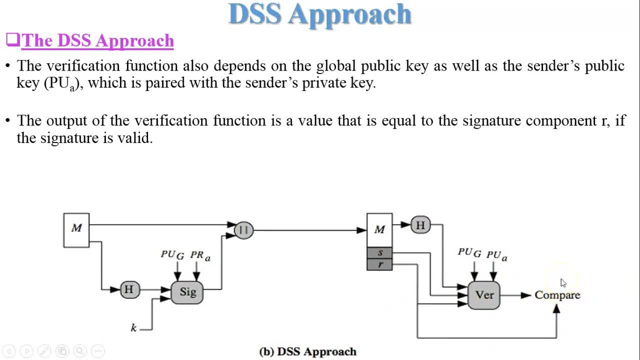 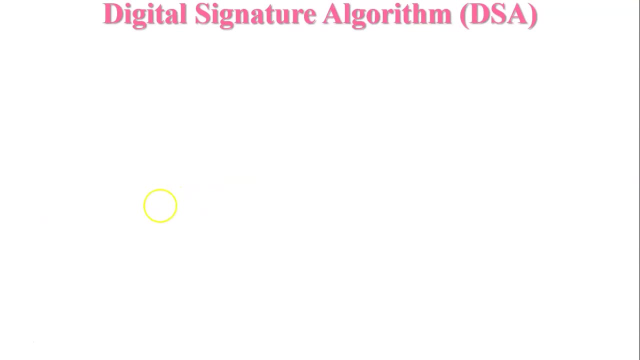 If both are same, it means message is valid and accepted by the particular receiver. The signature function is such that only the sender with knowledge of the private key could have produced the valid signature. Next, DSA: digital signature algorithm. So first step of any digital signature algorithm is key generation process. 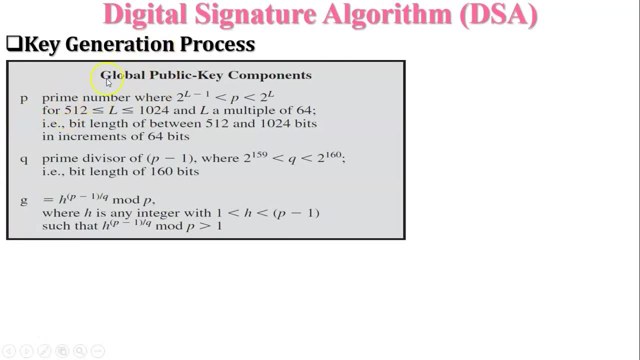 Now here, key generation process. there are, first of all, global public key component is used Here: P, Q and G. these three are The global public key component. Meaning of global public key component is: in network, all the users are connected with each other and the value of P, Q, G are the same for all the users in the network. 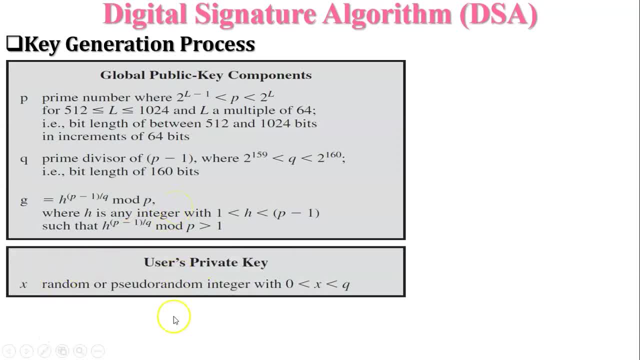 So it is called global public key component, Now user's private key, or we can say sender's private key, which is selected by the particular sender. Here X is the user's private key, Now user's public key. User's public key is calculated from the user's private key. 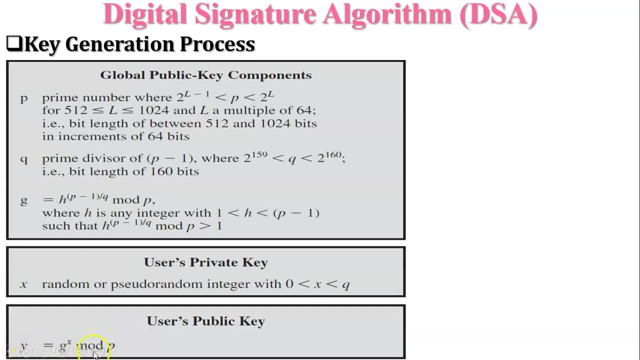 So now you can see over here from the equation: Y is equal to G raised to X mod P. Here X is the user's private key and G and P are the global public key component. Now this is the signing process, or we can say the sender side diagram of the digital signature algorithm. 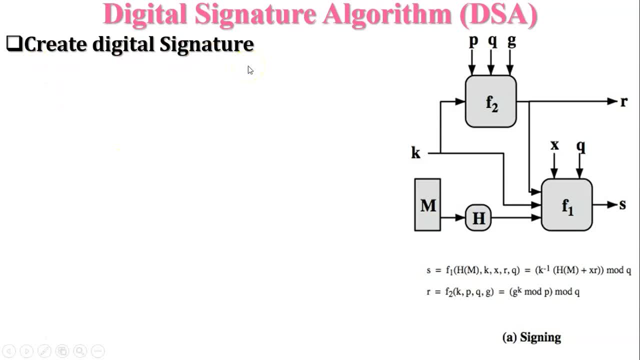 Now second step is create a digital signature. So how it creates. Now see first one Per message: secret number K. K is the random or pseudo random integer. The value of K is always different whenever your message is different, or we can say: new message is arrived. 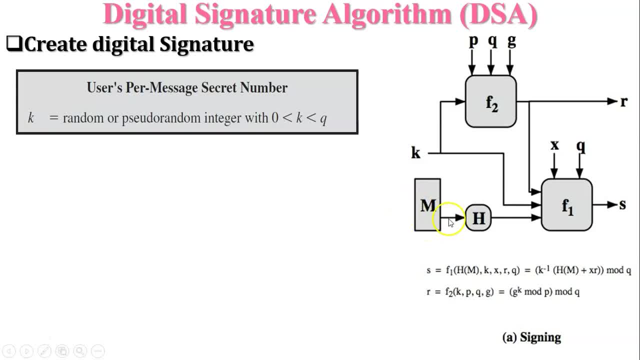 Now see in this figure From the message hash value is generated and input. output of the hash value, or we can say fixed hash value output is applied to the F1 function. Here different two component is generated: R and S. The combination of R and S is our digital signature, which is generated from the message. 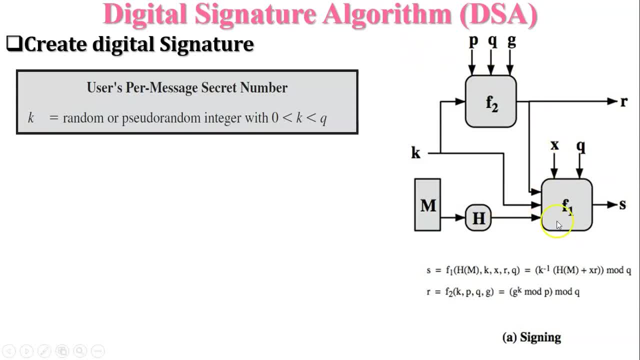 So discuss about F1.. Here input of the F1 is hash value, This is a per message secret number, and output of the F2 and user's private key X and Q is the global component of the users. Here F2 function is used. 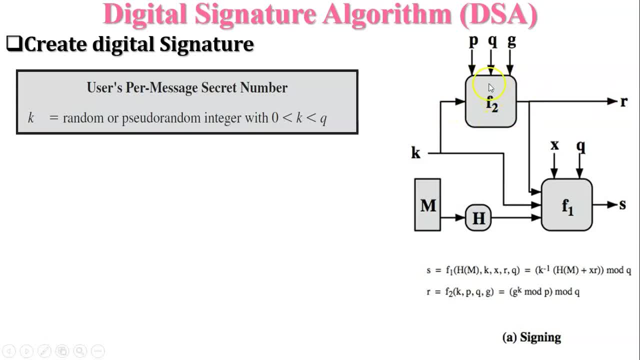 It generates R value. Input of the particular F2 function Is P, Q, G. This is the global components, or we can say global public key component, And the another input is K. This is users per message secret number. It generates R and it generates S. 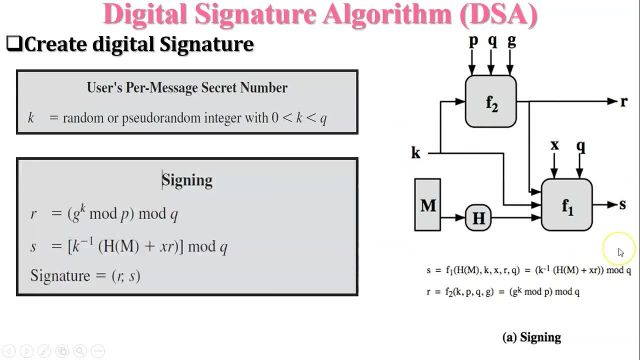 Here R and S is the, our final digital signature. So equation: R is equal to G, raise to key K mode P mode Q, and S is equal to K, inverse H of M plus X R mode Q. So the pair of this variable, R and S, is our digital signature. 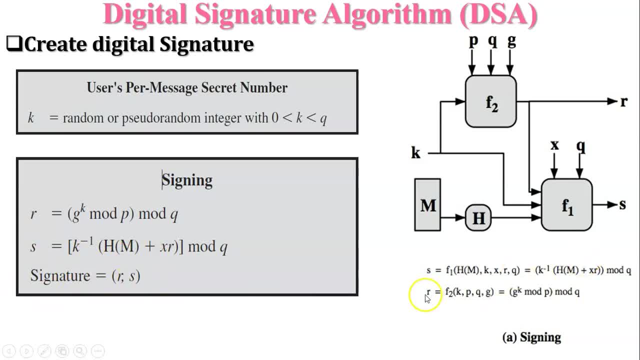 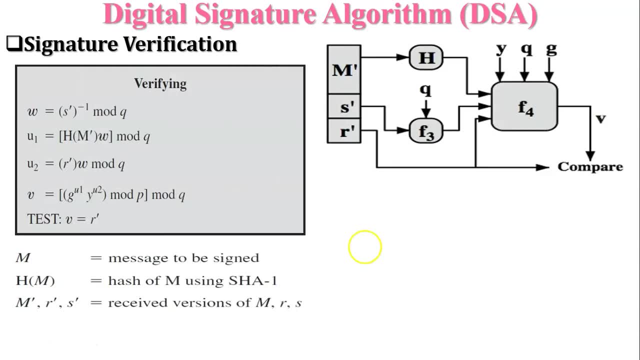 So signature is equal to R S and it is sent to the receiver side. So third process is signature verification at the receiver end. Now see in this figure: Here M dash, S dash and R dash are received. Here M is the message to be signed. 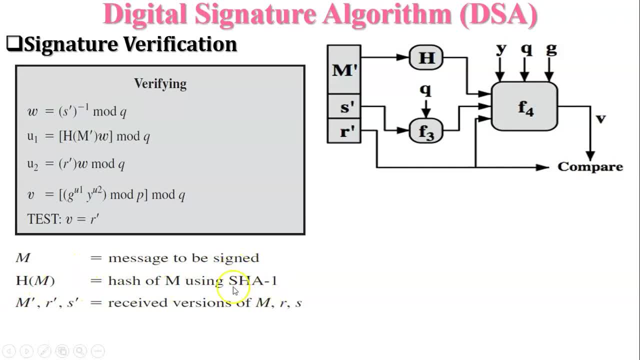 H of M is the hash value of the message. with the help of SHA-1 algorithm, M dash, R dash and S dash is equal to received M dash, R dash is equal to received version of M, R, S. So R and S is the, our digital signature component, and M is the message. 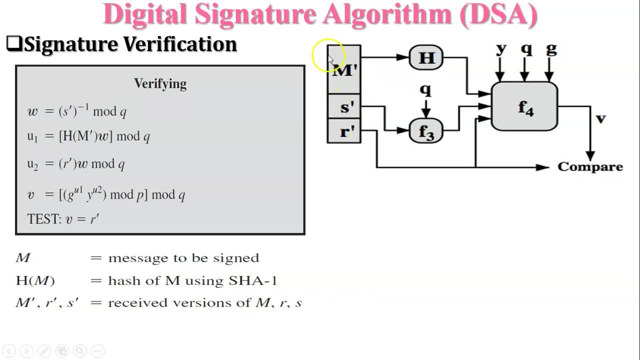 Now let us discuss about this diagram. From the M dash hash value is generated. So before discuss about F4 function, We will discuss about F3 function. Here, S dash is the input of the F3 function and Q. We can say this is the prime divisor. 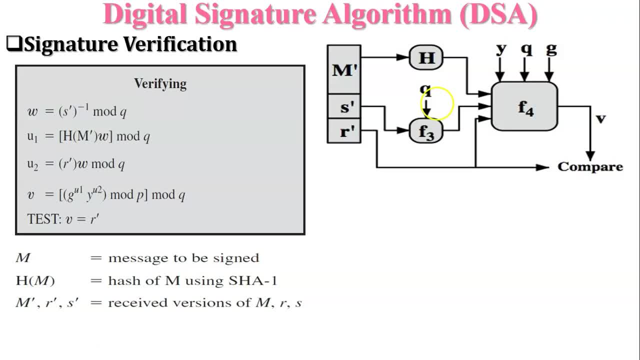 Or we can say Global public key component given to the F3 as input And the output of the F3 function. We can say it is W. Now you can see over here: W is equal to S dash minus 1 mod Q. 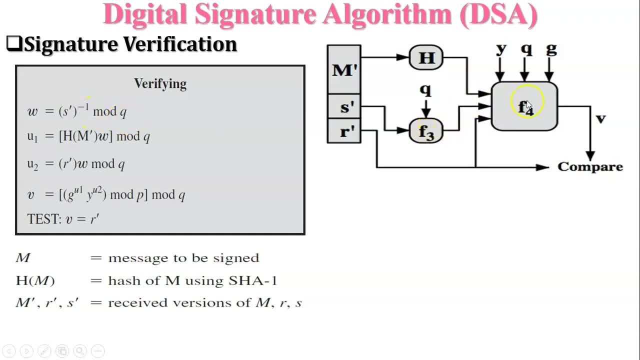 So output of the F3 is input of the F4. Now discuss about F4 function Here. output of the F4 is the V And V is the value which is compared with the R dash. If R dash and V, both are same, 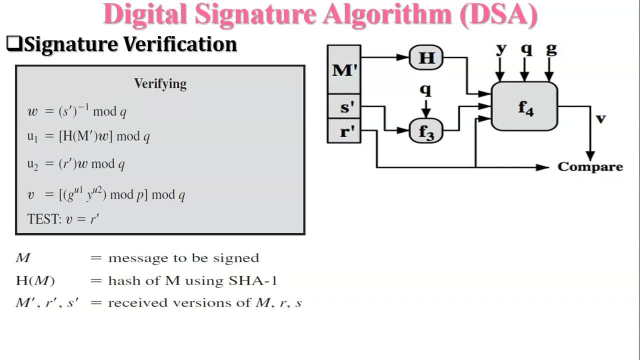 It means our digital signature is ok. There is no forgery in the signature. So how F4 will be generate Now. from the original message, Hash value will be generated and input to the F4.. Now Y is the public key of the sender. 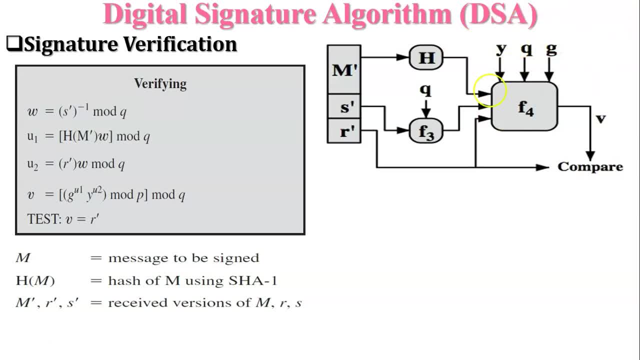 Here Q and G. both are the global public key component And another input is R. dash is given to the F4 and generate V. Now equation: V is equal to G. V is equal to G raise to U1.. G raise to U2. mod, P, mod Q. 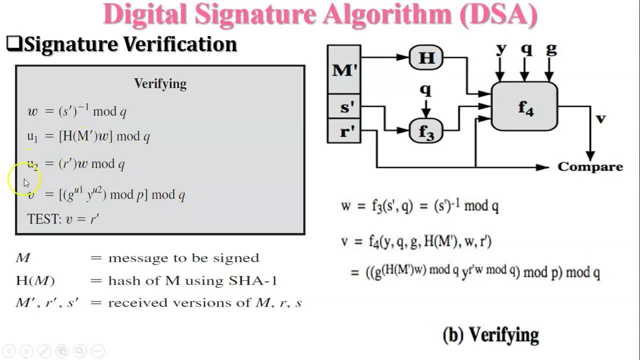 And U1. U2 is H of M dash W mod Q, And U2 is equal to R dash of W mod Q. So now here test, V is equal to R dash. If V is equal to R dash, It means our digital signature is valid.